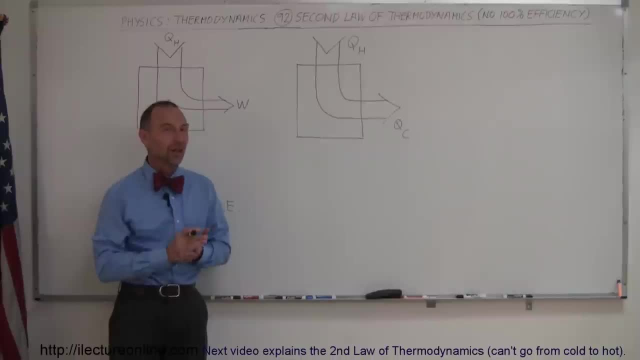 Here's our introduction on how to think about the second law of thermodynamics. Now, the first law of thermodynamics was a simple equation. It was simply: the change in internal energy of a gas equals the heat added to the gas, minus the work done by the gas. Very straightforward, so any 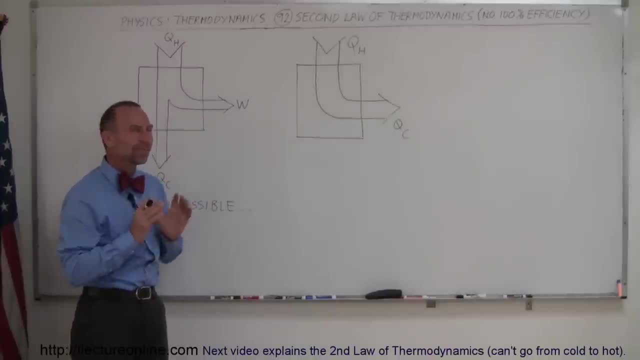 thermodynamic process. you knew that always to be true. But the second law of thermodynamics is not expressed in terms of an equation. It's expressed in terms of a concept. It's expressed in terms of what cannot happen in thermodynamics. So anytime we try to explain the second law of thermodynamics, 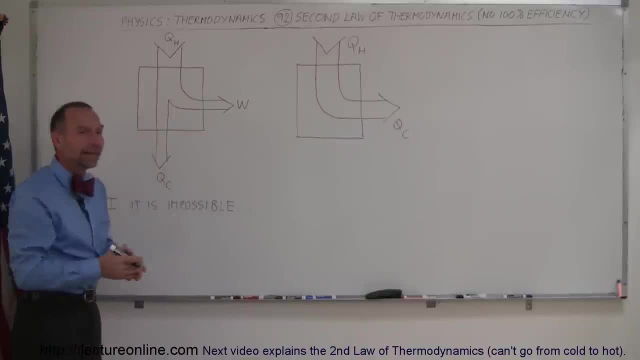 it should start with the words such as it is impossible, And it turns out that there's different ways in which to look at the second law of thermodynamics, Again to look at what is not possible. So the first way we're going to look at is in terms of the efficiency of an engine. 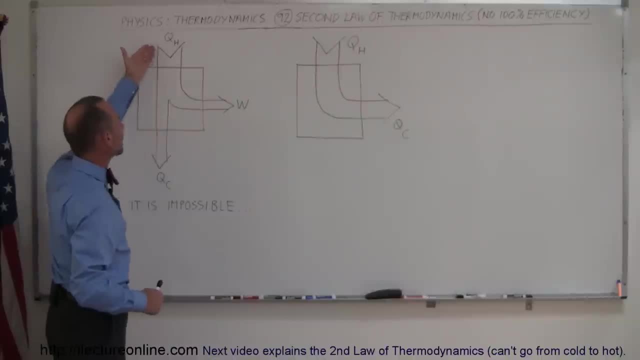 Like we said before, an engine works by extracting heat from a reservoir, taking part of that and making an engine work. so we can do work with the engine and then expelling some of the heat that was obtained from the hot reservoir into a cold reservoir or just simply expelling it exhausting. 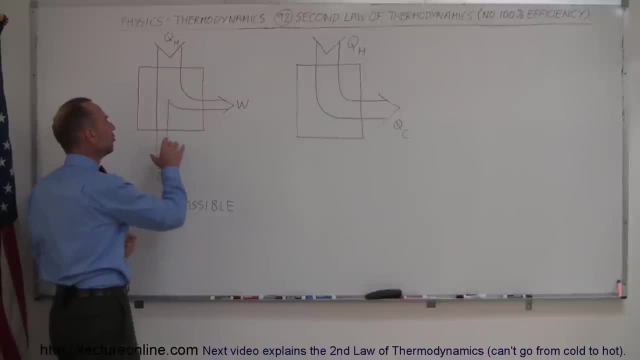 it And, as we expressed before, that the efficiency of an engine is simply a ratio of how much work we can do relative to the amount of heat that we extract. So again, we can write that the efficiency is simply equal to work divided by Q- hot, And of course, for that to be 100%, we want. 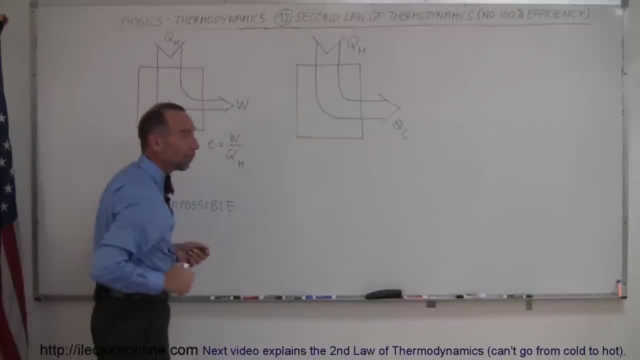 then all of the heat to be extracted from the hot reservoir and then we can do work with the engine. So we need to be used to do work. Example: what we have here to the right And it turns out in thermodynamics. 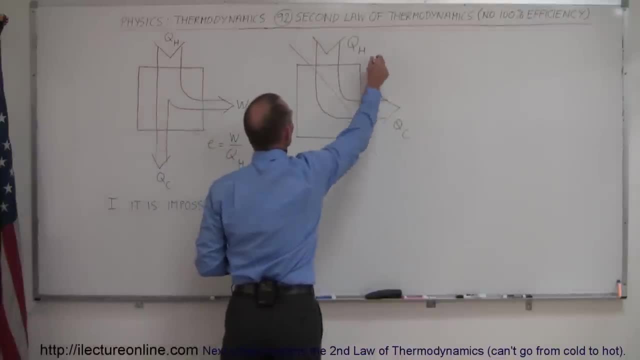 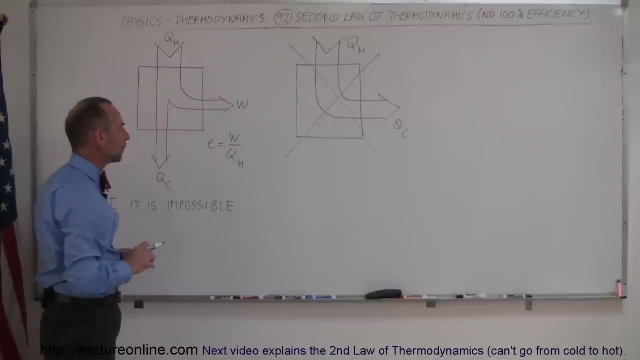 that is simply not possible. They say that it's not possible to extract all of the heat and use all of it to do work. So a way to look at that would be to have the different form of this equation. For example, we could say that: 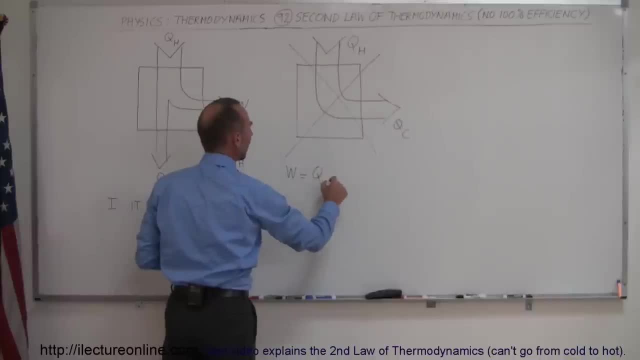 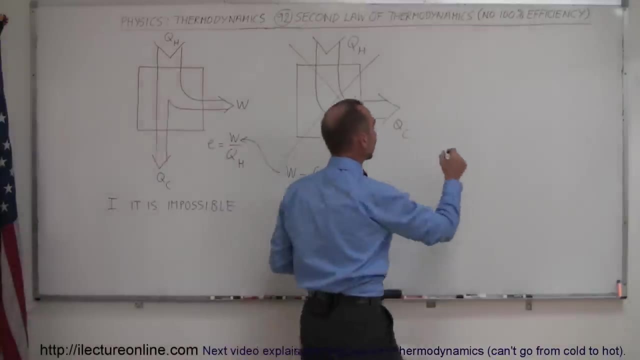 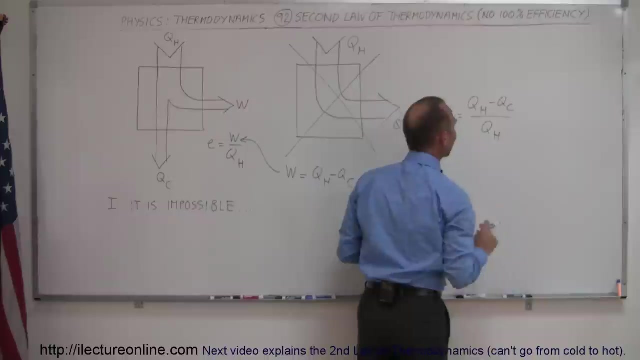 the work done by the engine is equal to Q hot minus Q cold. And if we replace the work in our equation there by that, we get the following: We get: the efficiency is equal to the difference Q hot minus Q cold divided by Q hot. And then the only way in which we can then get 100% efficiency,